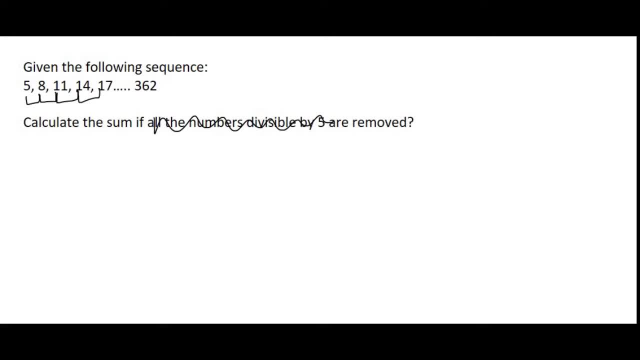 adding three each time, So we can work out the sum of the sequence by using the arithmetic formula for sums. So here we have been given the last term. So if you want, you could use this formula as well, but you don't have to. I usually just use this formula over here. 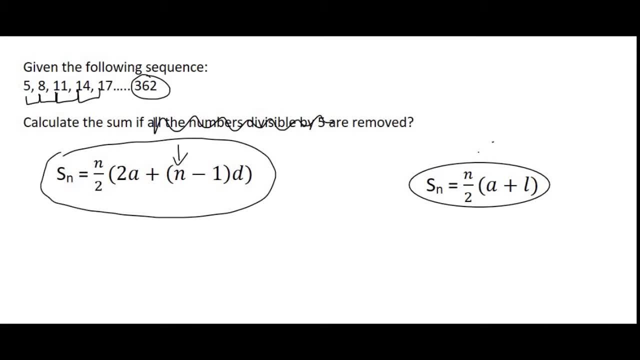 The only problem is is we don't know how many terms there are. So what I then do is I use the arithmetic term formula, which is the following: And we know that the last term has a value of 362.. The first term is five, The number of terms we don't know, And the common difference is three. 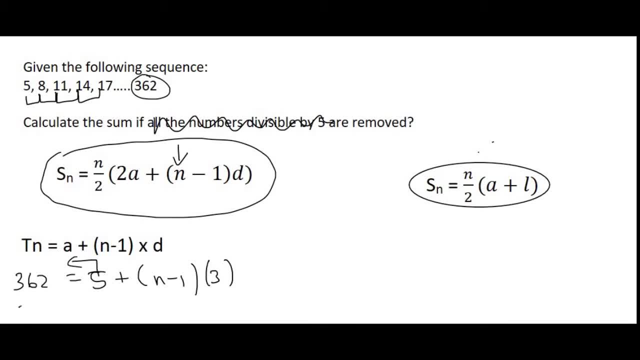 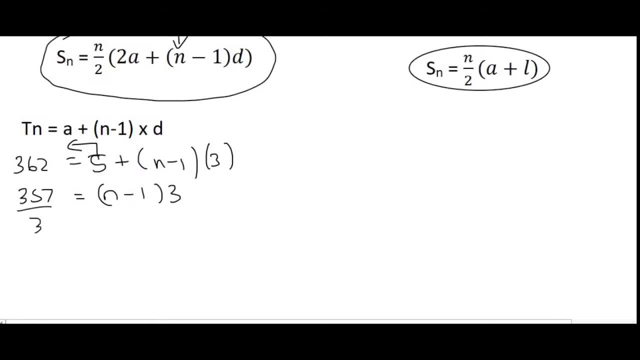 You then take the five over to the left, which gives you 357 equals to n minus one times three. You can then divide by three to get rid of this over here, Which gives us 119 equals to n minus one, And then, solving for n, you end up with 120.. So now we can. 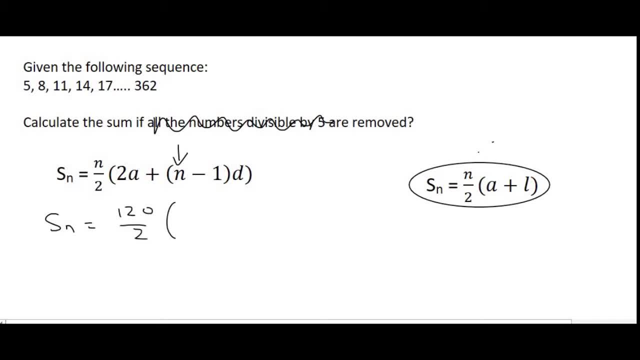 go work out the sum, because we know how many terms we have. So it's 120 terms. Term number one is five. 120 terms That's minus one, And then the difference is three. Then we can go calculate all of that And that'll give us 22,020.. Now, this formula would have been easier. 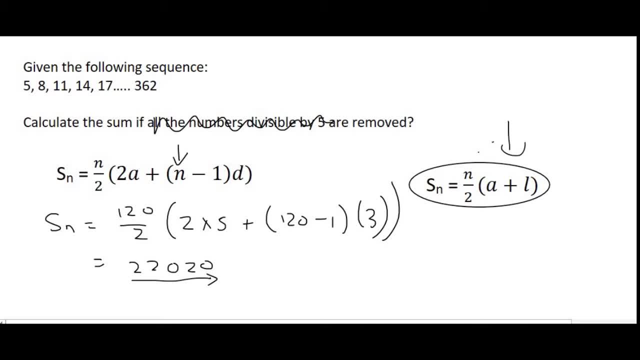 We would have just had. well, no, actually we still wouldn't have known what the number of terms were. So no, it wouldn't have been that much faster. So the sum of all of these numbers is 22,020.. We must just remember that. Now what we're going to do is take out all the numbers. 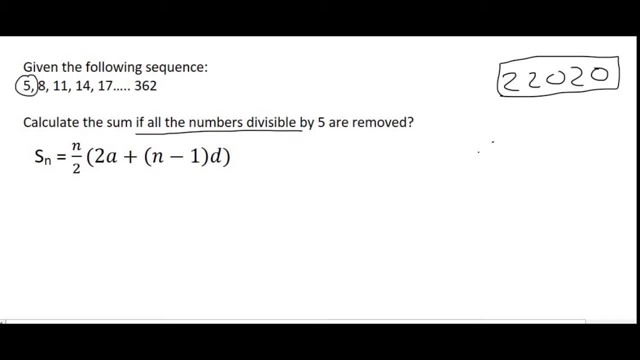 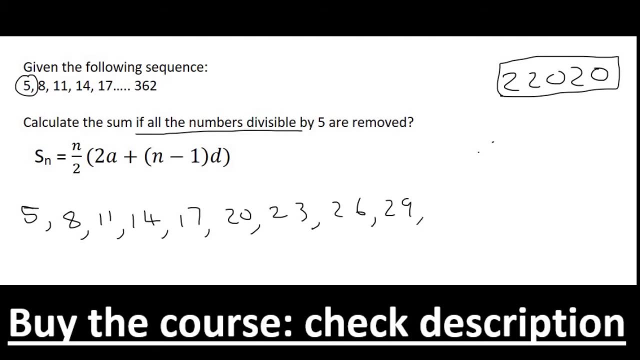 that are divisible by five. So that's going to be this five in the beginning. Then what I'm going to quickly do is just carry on the sequence quickly: 11,, 14,, 17,, 18,, 19,, 20.. Next would be 20.. Then there would be 23,, 26,, 29,, 32, and 35. We need to look for at. 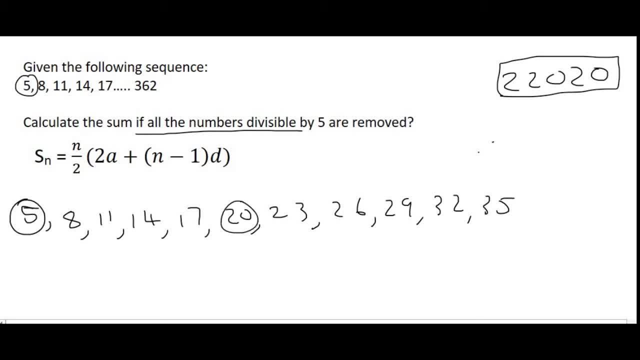 least three numbers that are divisible by five. So we have five, 20, and 35. We're now going to take those out of the pattern, So we'll just have five, 20, and 35. And we hope, and it's always- 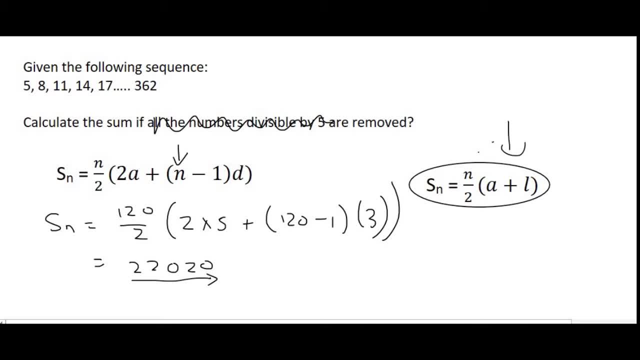 We would have just had. well, no, actually we still wouldn't have known what the number of terms were. So no, it wouldn't have been that much faster. So the sum of all of these numbers is 22,020.. We must just remember that. Now what we're going to do is take out all the numbers. 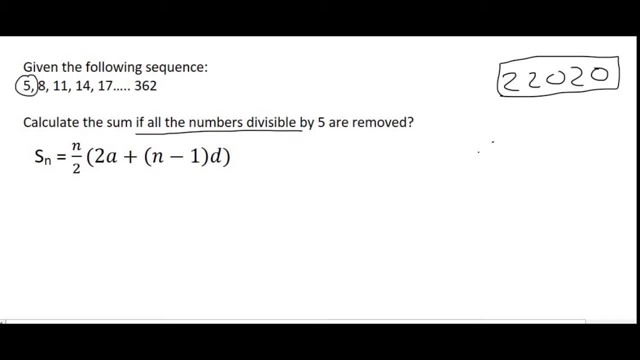 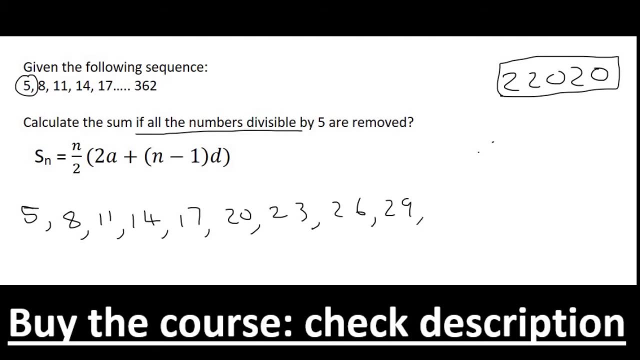 that are divisible by five. So that's going to be this five in the beginning. Then what I'm going to quickly do is just carry on the sequence quickly: 11,, 14,, 17,, 18,, 19,, 20.. Next would be 20.. Then there would be 23,, 26,, 29,, 32, and 35. We need to look for at. 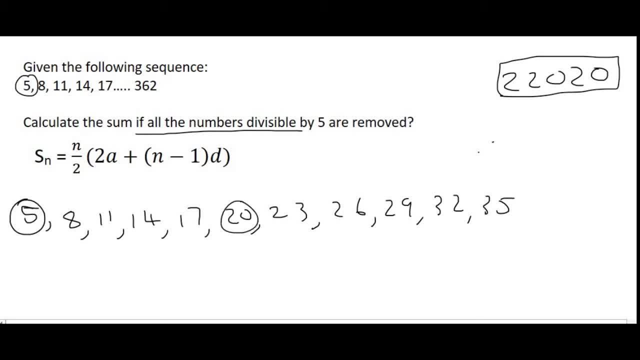 least three numbers that are divisible by five. So we have five, 20, and 35. We're now going to take those out of the pattern, So we'll just have five, 20, and 35. And we hope, and it's always- 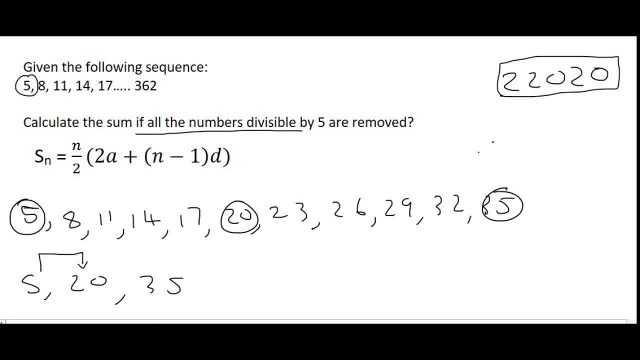 going to work out. these numbers should form their own pattern, And they do, So we're going to add 15.. Notice that you have to add 15 each time, So this becomes its own little arithmetic formula. So we could simply go and calculate the sum of that. However, we don't know what the last term 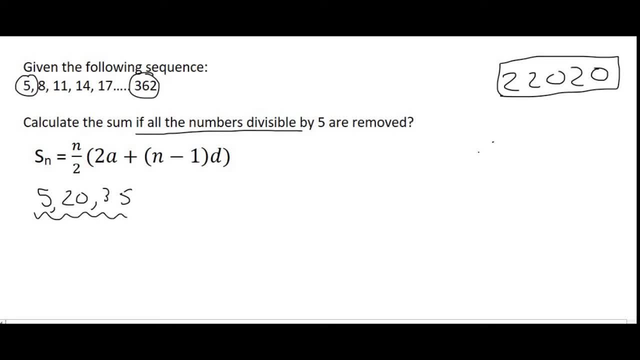 in our sequence would be: It's not the 362, because that's not divisible by five, Because right now we are trying to look at the terms that are divisible by five. So what we do is we go from the 362 and we work our way backwards in the original sequence, because we know that the 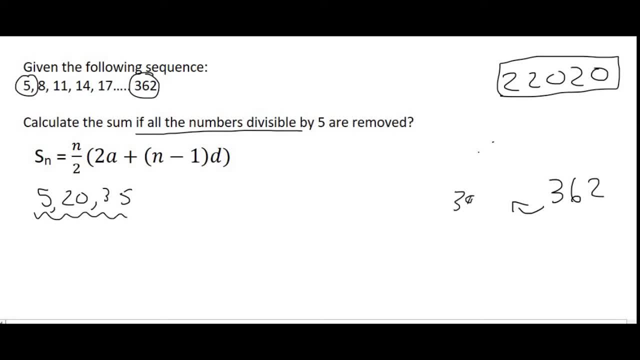 difference is three, So we're going to add 15.. And we're going to add 15. And we're going to minus three, then the previous number should be 359,, then 356,, then 353,, and then 350,, which is 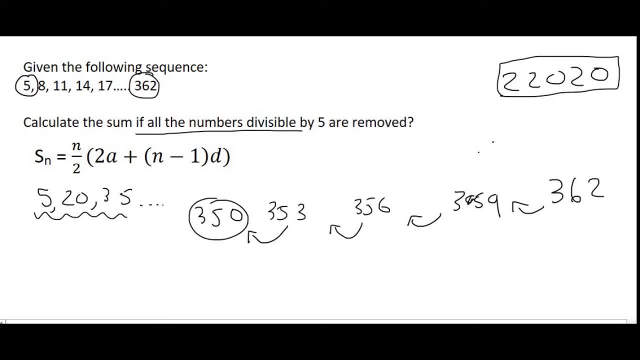 divisible by five. So the last term in our divisible by five pattern is 350.. So then, what we can use is use the term formula for arithmetic to work out how many terms we have in that pattern over there, where the last term is 350.. 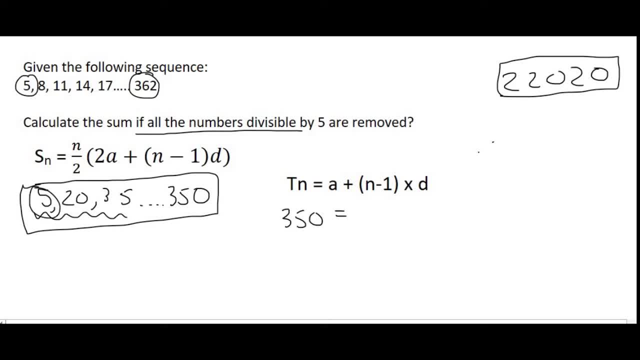 A is going to be five. Remember, we're not looking at the original sequence anymore, We're just looking at this one, And the common difference is not going to be three, like it was over here, but rather 15.. Can you see, we're adding 15 each time, So now we can take the five over to the 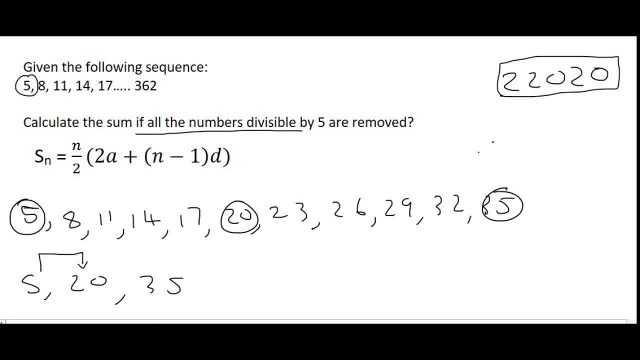 going to work out. these numbers should form their own pattern, And they do, So we're going to add 15.. Notice that you have to add 15 each time, So this becomes its own little arithmetic formula. So we could simply go and calculate the sum of that. However, we don't know what the last term 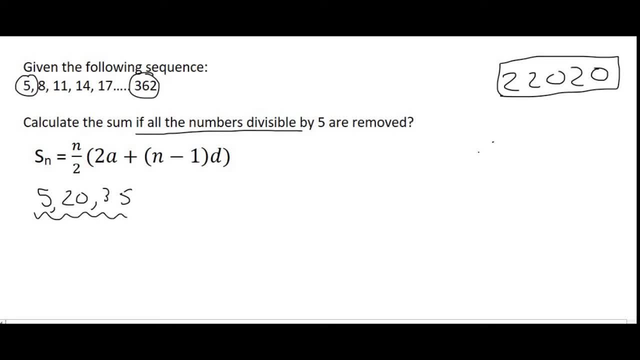 in our sequence would be: It's not the 362, because that's not divisible by five, Because right now we are trying to look at the terms that are divisible by five. So what we do is we go from the 362 and we work our way backwards in the original sequence, because we know that the 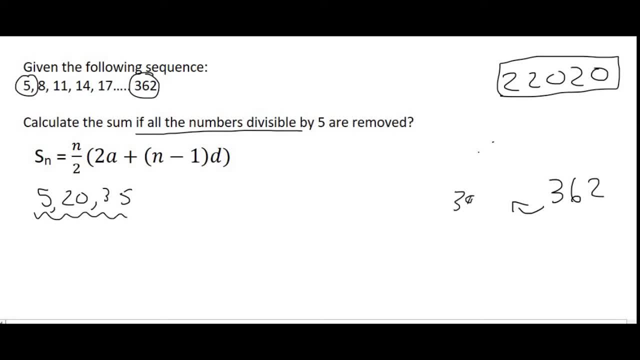 difference is three, So we're going to add 15.. And we're going to add 15. And we're going to minus three, then the previous number should be 359,, then 356,, then 353,, and then 350,, which is 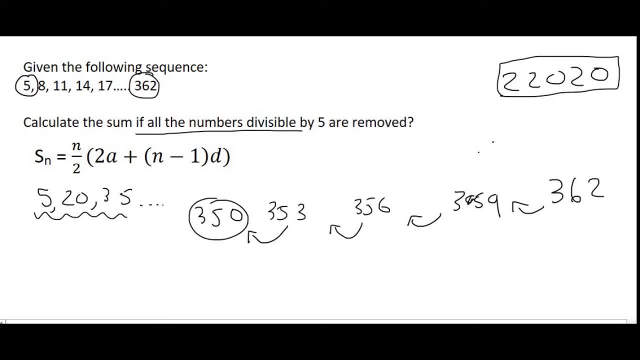 divisible by five. So the last term in our divisible by five pattern is 350.. So then, what we can use is use the term formula for arithmetic to work out how many terms we have in that pattern over there, where the last term is 350.. 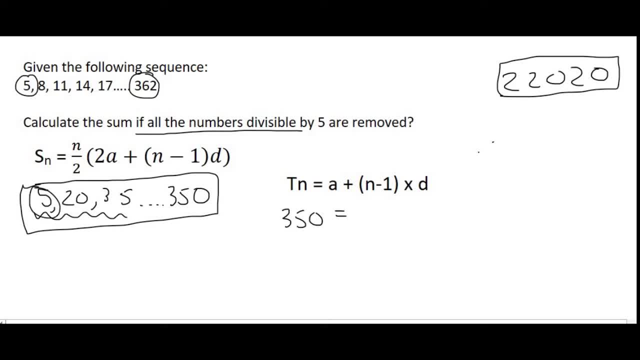 A is going to be five. Remember, we're not looking at the original sequence anymore, We're just looking at this one, And the common difference is not going to be three, like it was over here, but rather 15.. Can you see, we're adding 15 each time, So now we can take the five over to the 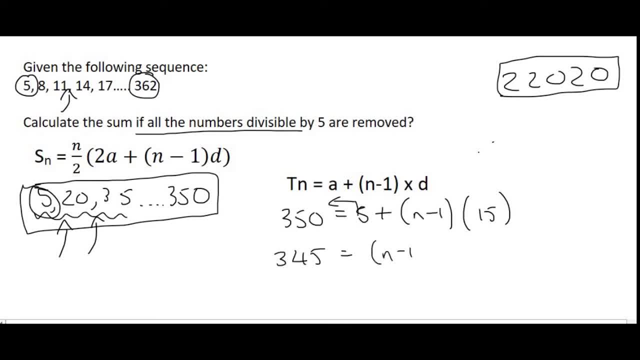 left. That's 345 equals to n minus one times 15.. We can then divide by 15 on the left hand side, And that'll give us 23 equals to n minus one. And then we start to work our way back to the. 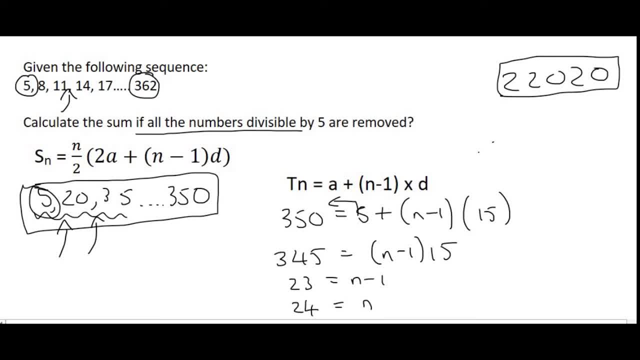 so for n we get 24 terms. So there are 24 terms that are divisible by five. So we now know that there are 24 terms in the divisible by five pattern, And so we can calculate the sum of those 24 terms by using the sum formula. So it's 24 terms over to two times a, which is five. 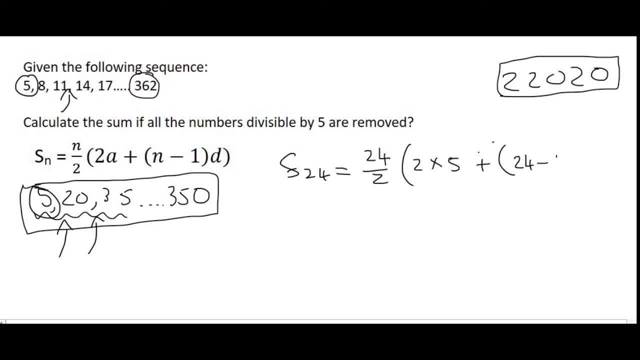 plus, the number of terms is 24 minus one, And the common difference in that pattern is now 15.. It's not the 3 that we have in the original pattern, it's 15.. So we go ahead. we type that all in on the.